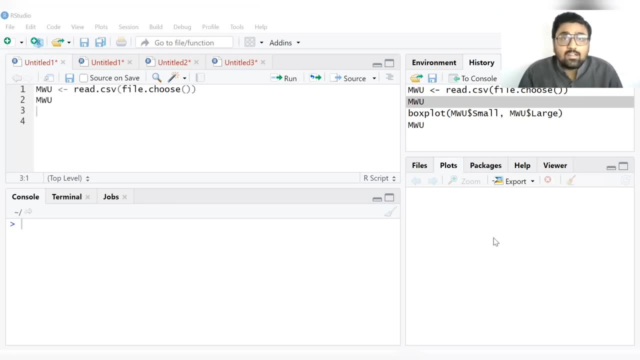 these two groups. So here we have two independent groups. Group 1 consists of people live in small cities and group 2 consists of people live in large cities. Now, what is the null and alternative hypothesis in this case? The null hypothesis says that the data from large and small cities are 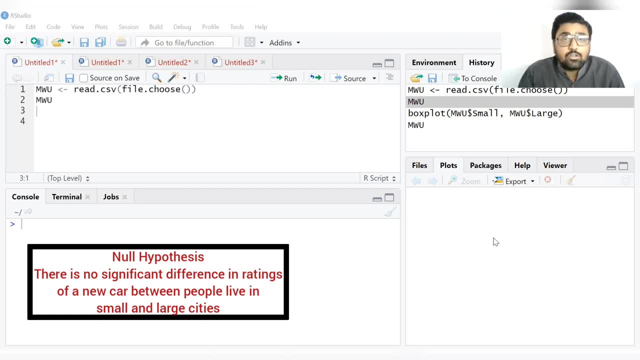 not significant. So in this case there is no significant difference in the ratings of a new car between people live in large and small cities, against the alternative hypothesis of a significant difference. Now let's understand the data. So here we have MWU data, that is, Mann-Whitney U-Test. 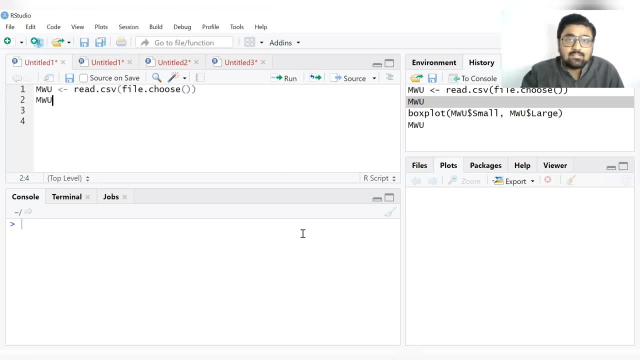 I have already inserted the data from CSV file to RStudio. If I run this, you can see the data. So we have data from 10 people live in small and large cities and their ratings on a 0 to 10 scale regarding the new car. Now, before we perform the Mann-Whitney U-Test, we can visualize. 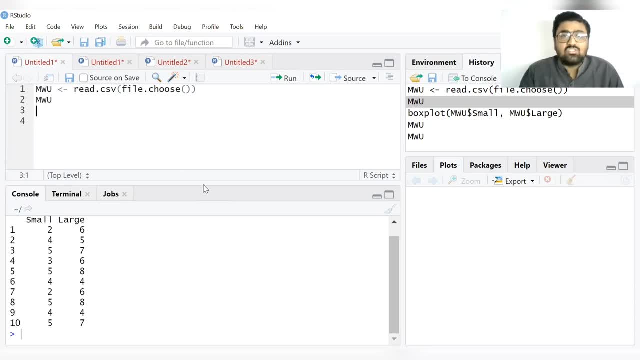 the data with the help of box plot. So let's generate the box plot. To do so, we have the option of box plot, MWU. That is our data. Mann-Whitney U-Test dollar, small and large. Simply click on run, Sorry. 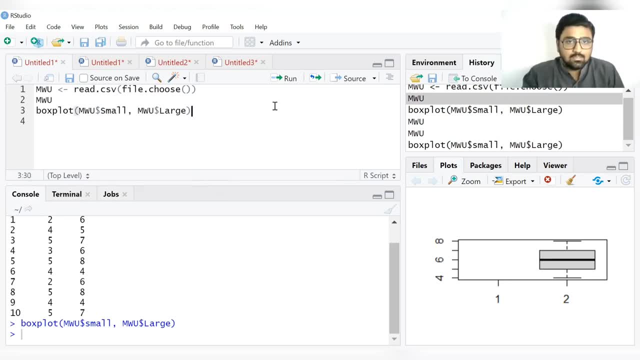 here we have capital S. So you can see the box plot of the ratings of people live in small and large cities. So you can see the box plot of the ratings of people live in small and large cities regarding the new car. Now to perform Mann-Whitney U-Test, we have the command called: 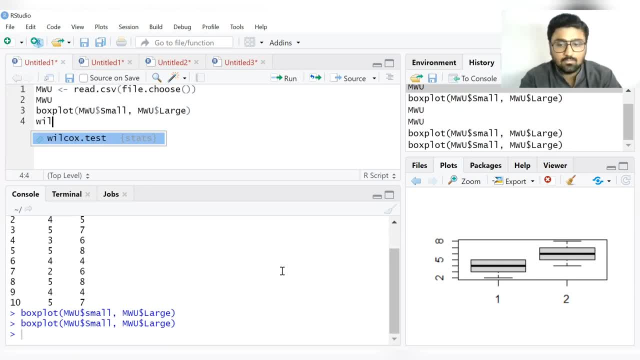 Wilcox-Test. So here first we write the group 1.. So our group 1 is small, group 2 is large, which means that we are comparing these two groups. Now write: confidence interval is equal to true. So that will generate the confidence interval for our confidence level. So define.